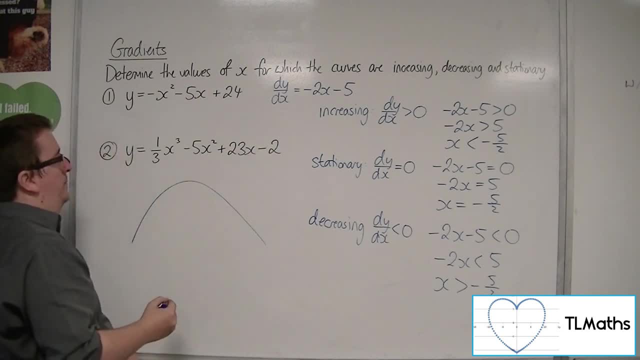 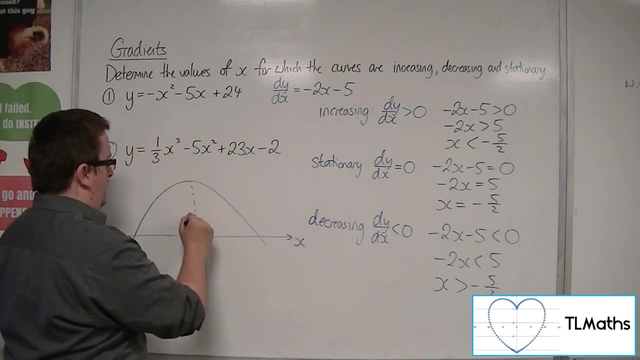 I could think: well, that's a graph that's going to look like this. So if I draw in an x-axis that's minus 5 halves, I don't care where it's crossing the x-axis. that's not interesting to me. 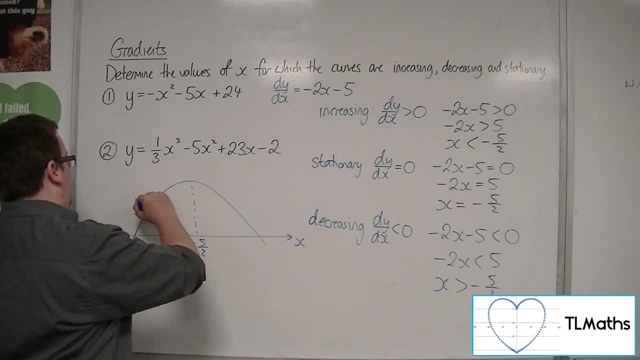 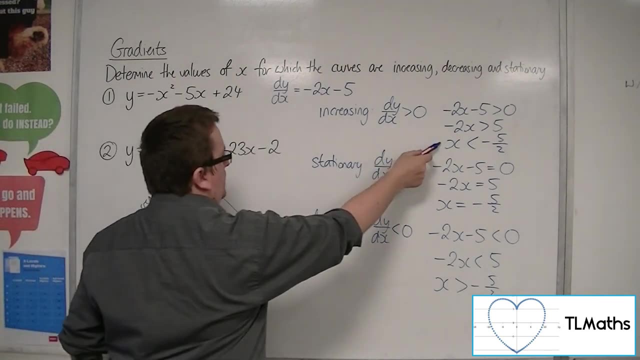 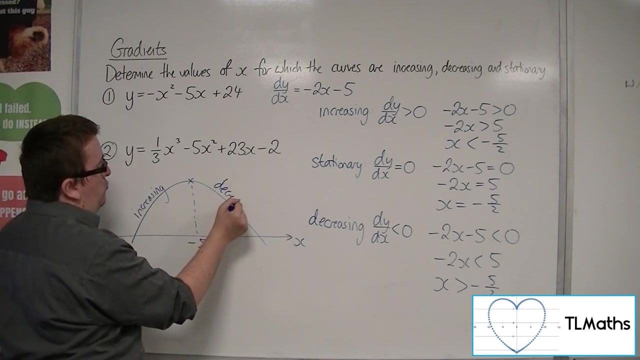 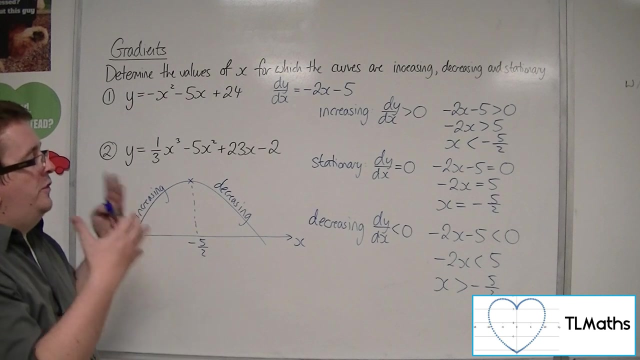 But I do know that we are increasing here. so when x is less than minus 5 halves, I know we're stationary at minus 5 halves and I know we are decreasing when x is greater than minus 5 halves. So as long as I've found the stationary point, 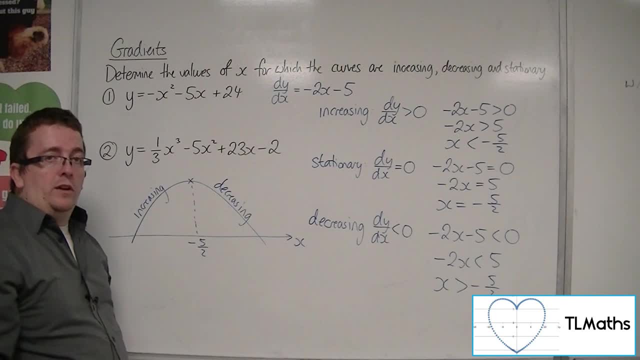 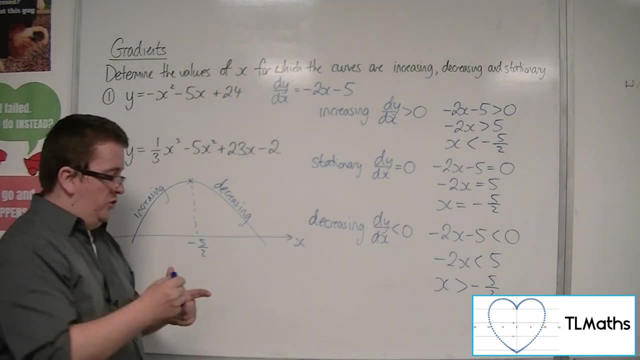 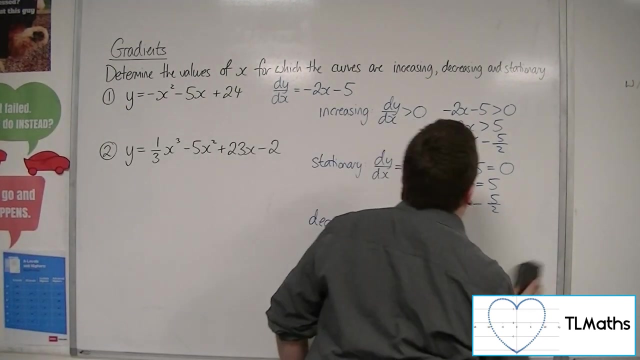 I can then draw a little graph of what this would look like, to then identify the inequalities. But doing it algebraically works just as well. So let's have a look at number 2.. I'll get rid of that and that as well. 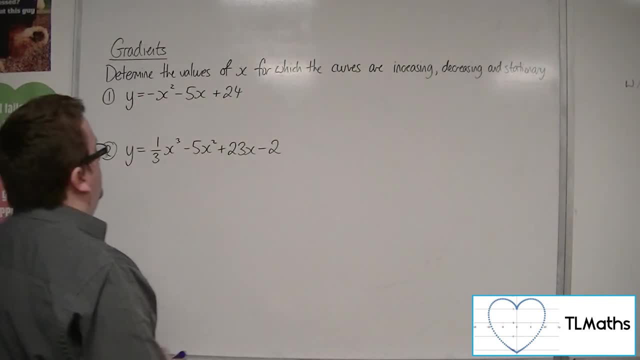 Okay, So first of all the y by the x. So, differentiating this, I'm going to get the 3 multiplying with the 3rd, so x squared. take away 10x plus plus 23.. 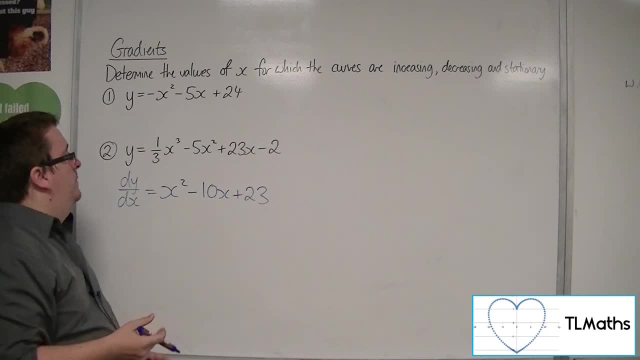 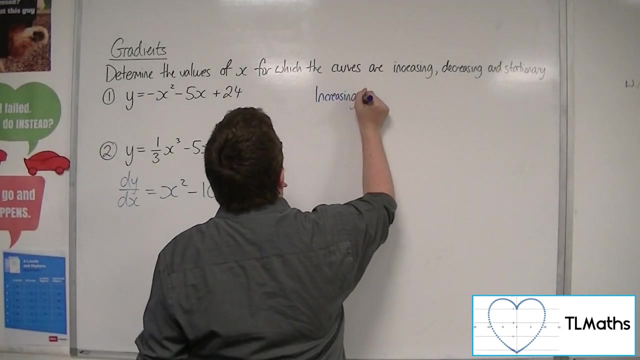 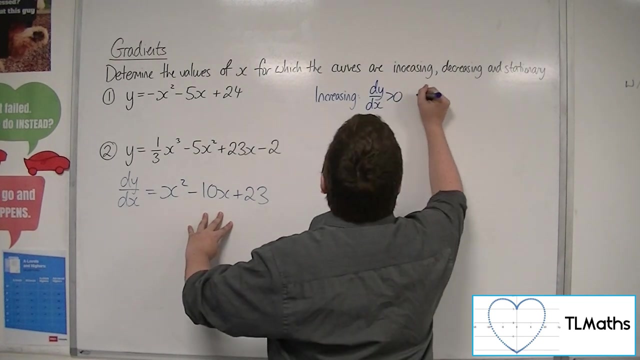 Okay Now if I use the same technique as I did before, okay with number 1, then what I'm looking for is if it's increasing. I want to solve the inequality. dy by dx is greater than 0.. So x squared minus 10x plus 23,. 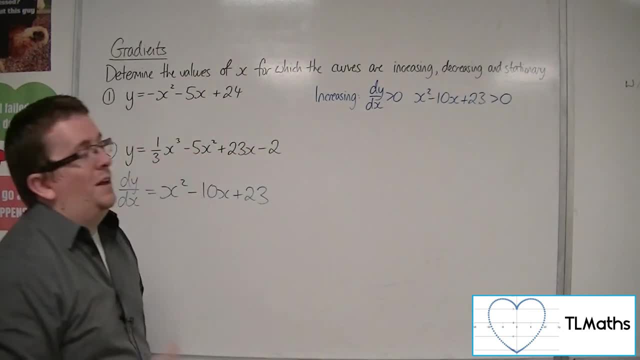 is greater than 0.. But I'm going to need to figure out where that curve crosses the x-axis. So really I want to solve the stationary points bit first. Okay, So stationary, when dy by dx is equal to 0.. 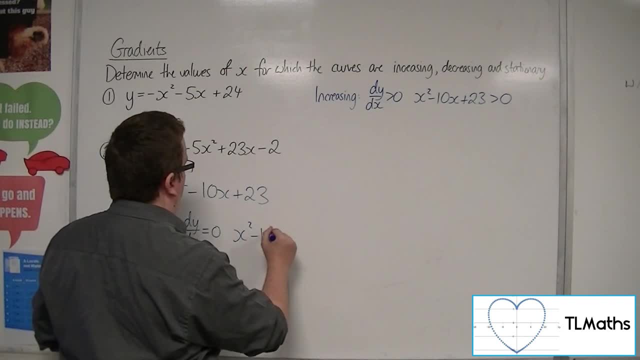 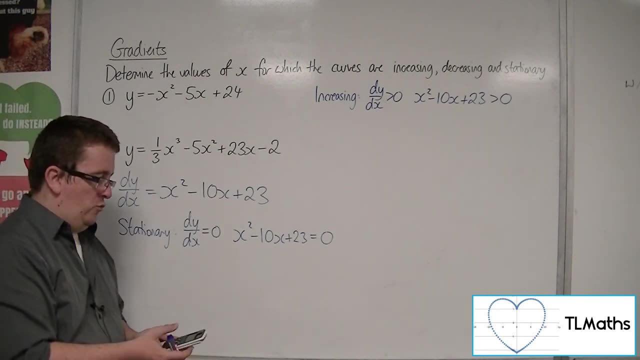 So x squared minus 10x plus 23 is equal to 0.. Now that doesn't matter. That doesn't look like it's going to factorise. So if we use the quadratic solver on our calculator, we can get 1 minus 10, 23.. 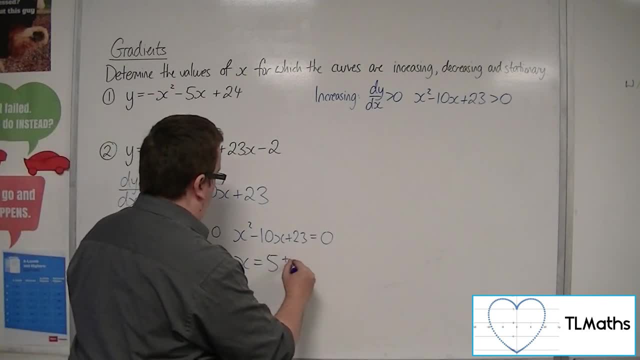 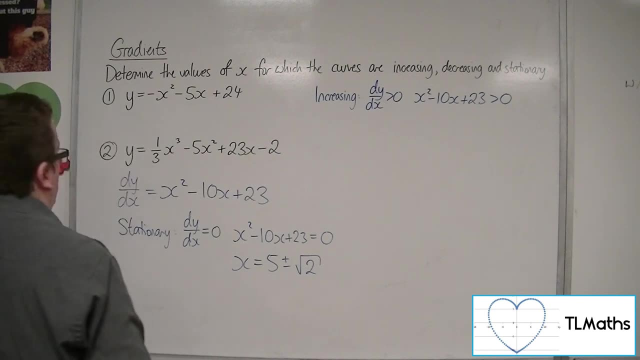 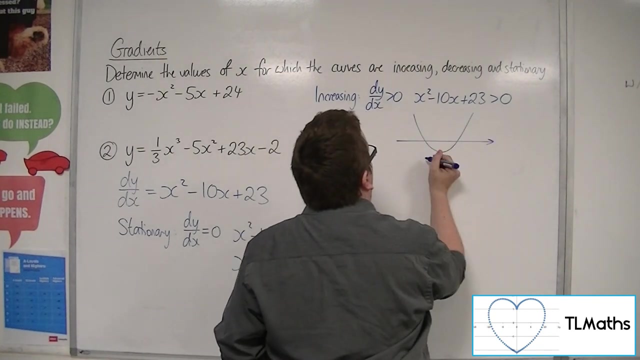 So 5 plus or minus root 2.. Okay, They're the solutions to that quadratic. So to solve that, I'd be looking at where this parabola is above, above the x-axis. So we'd have 5 minus root 2 here. 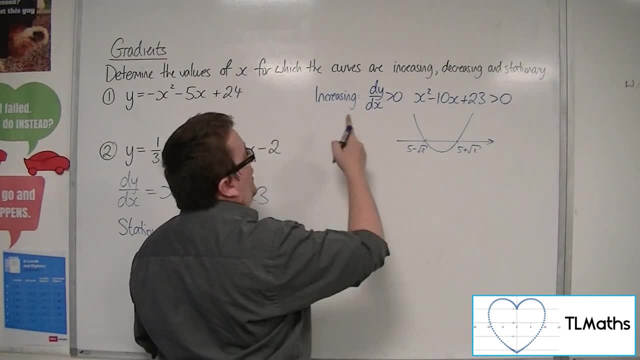 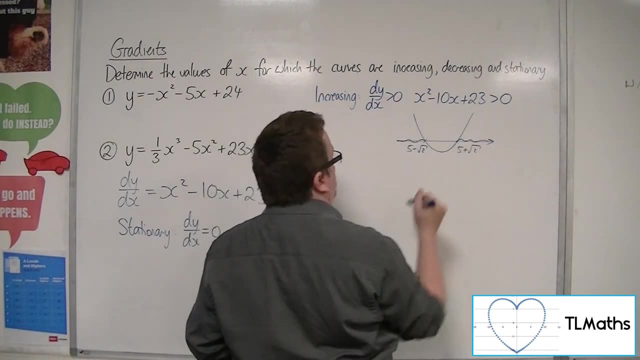 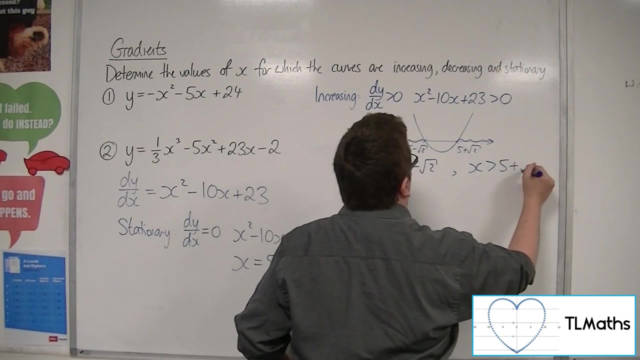 5 plus root 2 here. So it's increasing when we're above the x-axis. So in this region and that region, So x is less than 5 minus root 2, and x is greater than 5 plus root 2.. 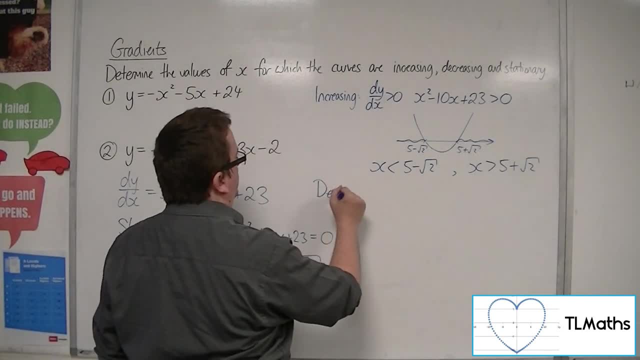 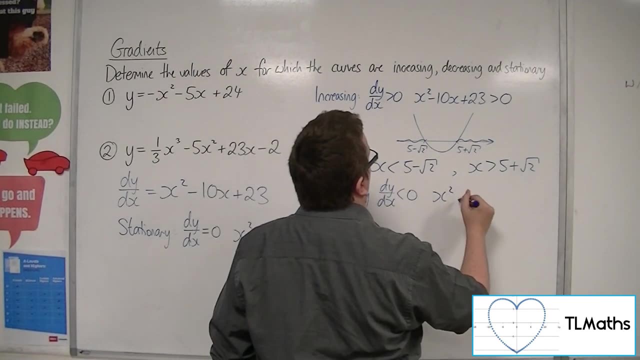 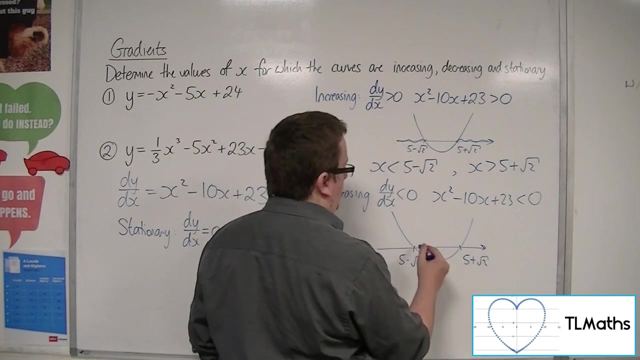 So we'd be decreasing, decreasing, decreasing, decreasing when dy by dx is less than 0. So solving the inequality x squared minus 10x plus 23 is less than 0.. So, in other words, where is the parabola now below the x-axis? 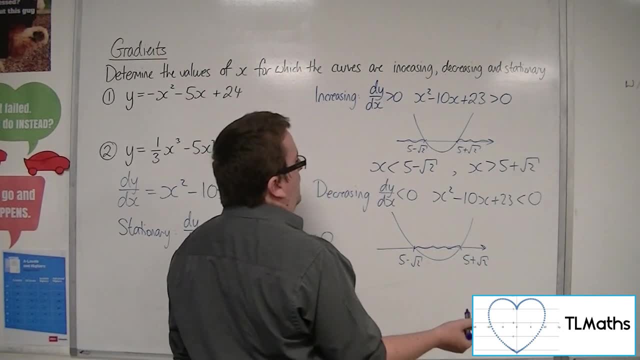 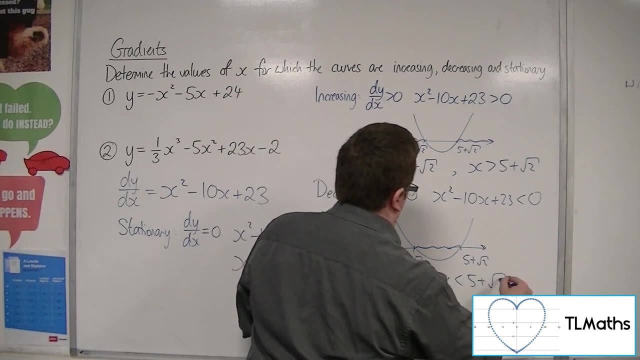 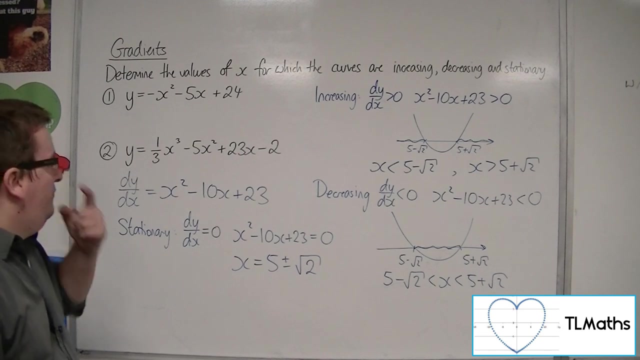 So it's below it there. Okay, So we'd be between these two values. Now can we visualize what's going on here? Okay, so really what's happening is that you've got some parabola- Sorry, not parabola, but a cubic curve here. 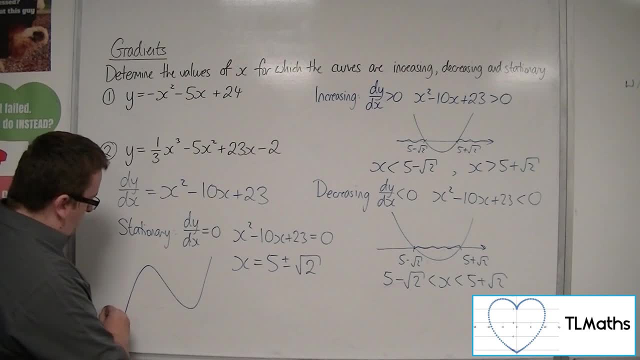 Okay, it's got its two stationary points. Now I don't know kind of, where it sits on the x-axis, I don't care. okay, where it's crossing the x-axis, Don't care about that. That point is representing your 5 minus root 2.. 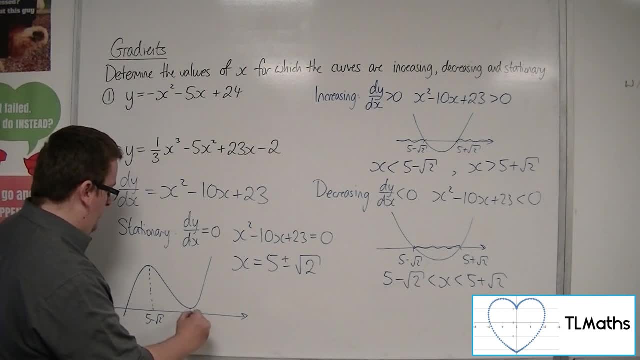 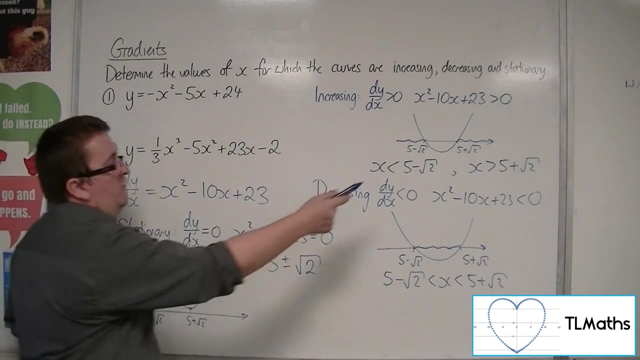 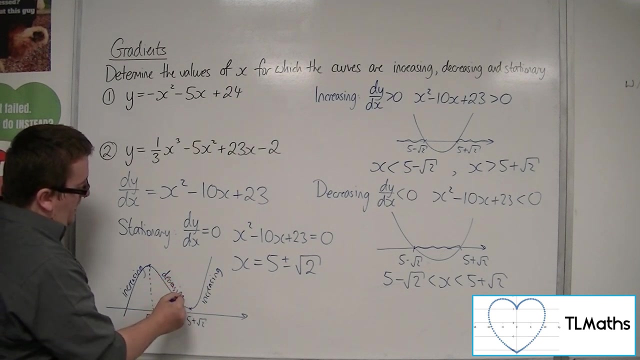 That point is representing your 5 plus root 2.. There's your stationary points. So it's increasing when x is less than 5 minus root 2.. And it's increasing here when x is greater than 5.. And 5 plus root 2 is decreasing between those two values.